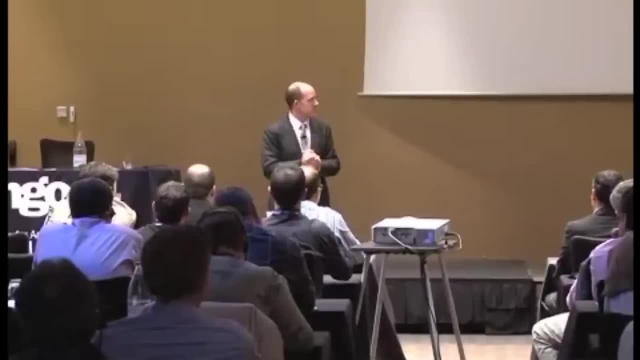 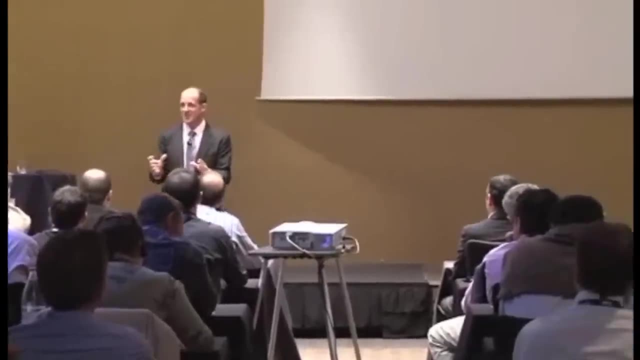 my name is Connor Neal, I'm from Tango and this talk is about the latest trend in monitoring strategies. Now, all of you are sitting with a piece of paper in front of you that says I'm Connor Neal, I've come from Ireland and I'm going to talk about Tango 04 and this. 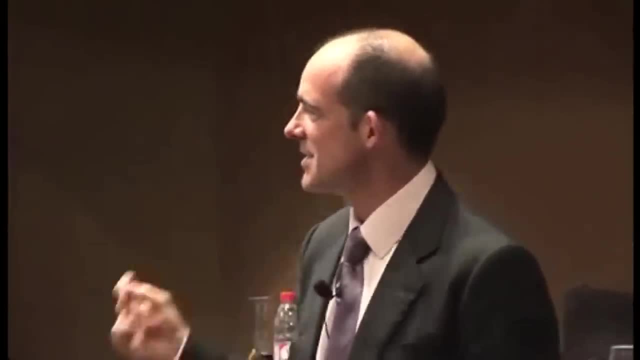 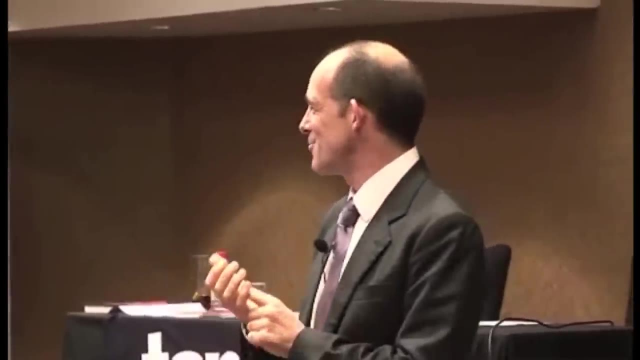 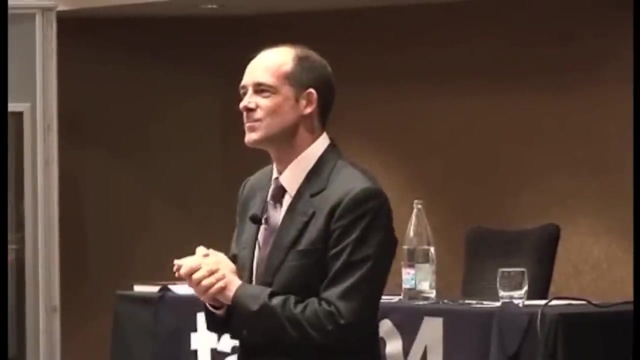 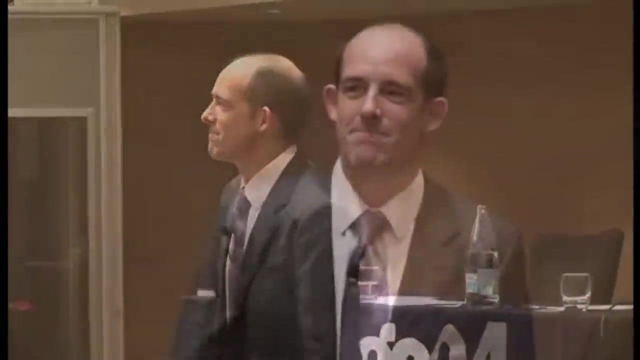 So by repeating what you already know, I'm giving a signal that it's a time to get your BlackBerry out. I've just signaled that this talk is opportunity to reconnect with BlackBerry. make sure the office is okay. Maybe get some plans together for the weekend. Another way to start: The lights, the mic's. 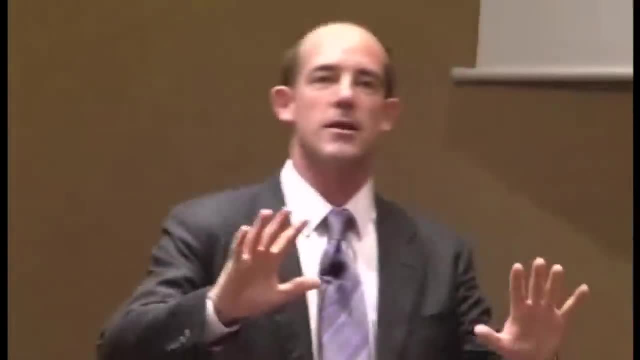 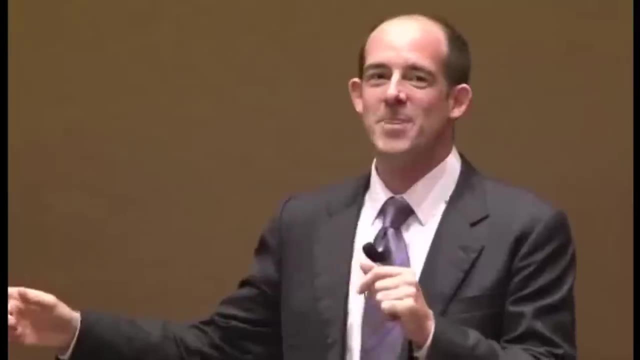 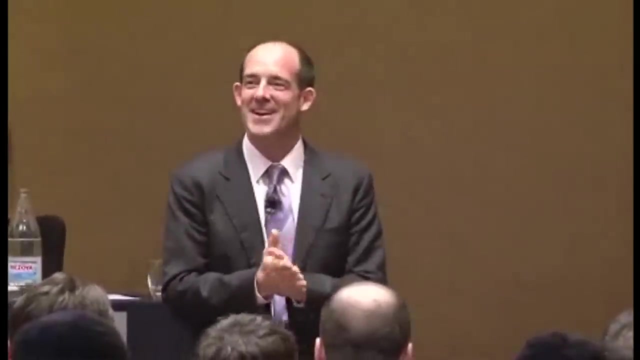 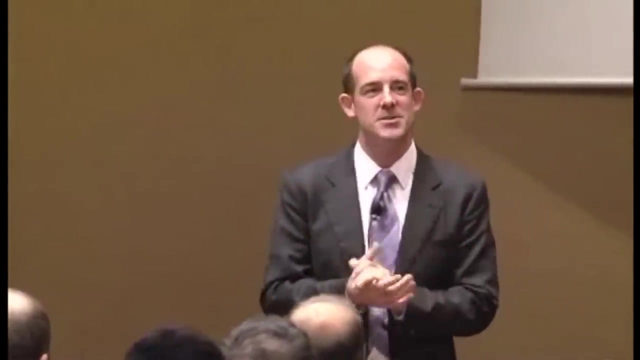 working. How much time have I got Okay, Right, Okay, Is it plugged in? And you laugh. but I guarantee tomorrow There's going to be some moments that get a little bit of that. And why? Because this is, for some of you, the first time you see this individual. they're here as a leader. 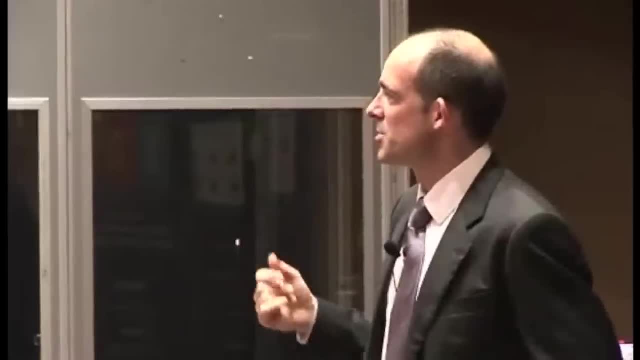 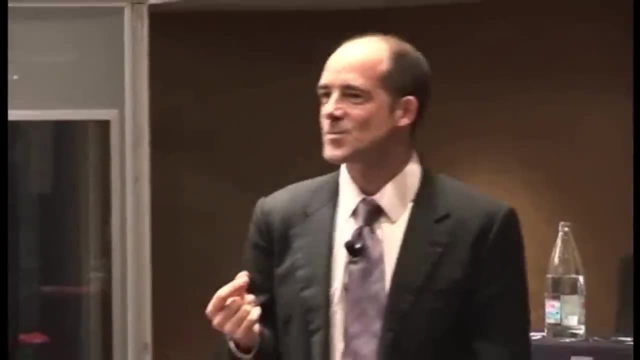 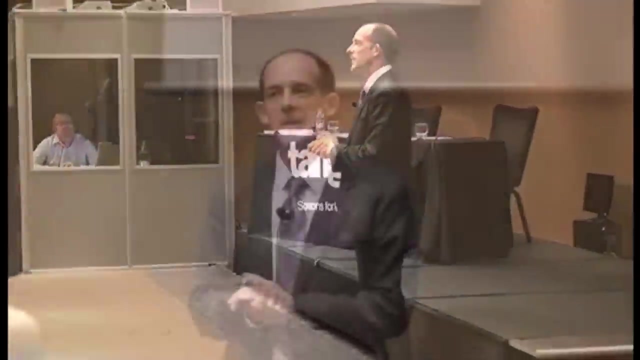 in their industry And your kid at school presenting on giraffes does a better job. That's sad, So I think there's only three ways of starting a speech. ** nytj aqueles angusakesment, Hanif puegarw. hi, I'm Connor Neal. I'm Irish, age 38, much like you were before you walked. 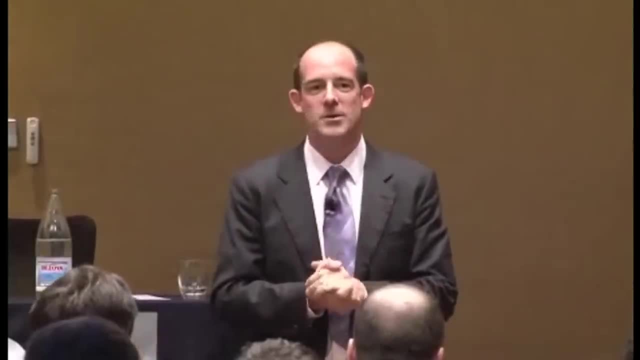 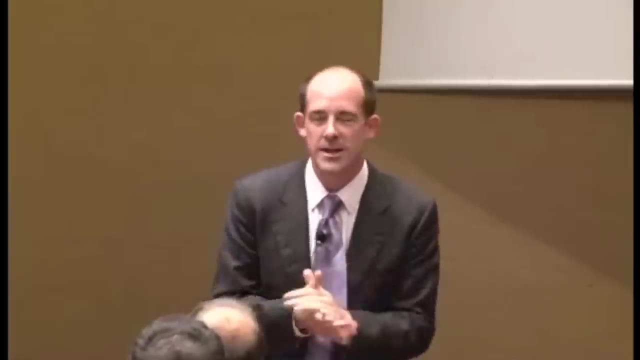 into this room and maybe I came up to a group, this group of 3 people who are having a little conversation. I walk in and I say: hi, I am Connor, I am Irish, 38-years-old, I have a interest in sailing, I like running, and they've walked away. 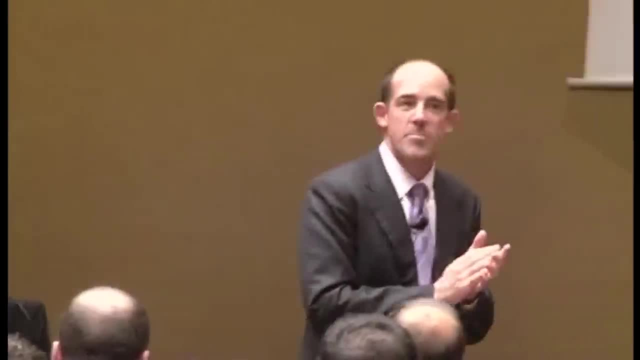 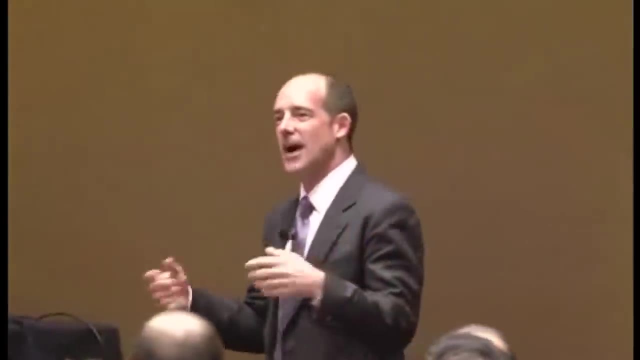 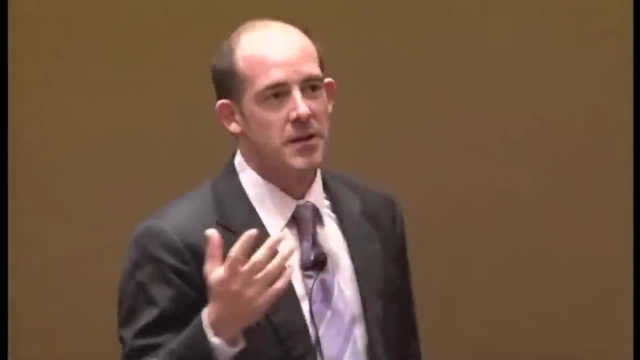 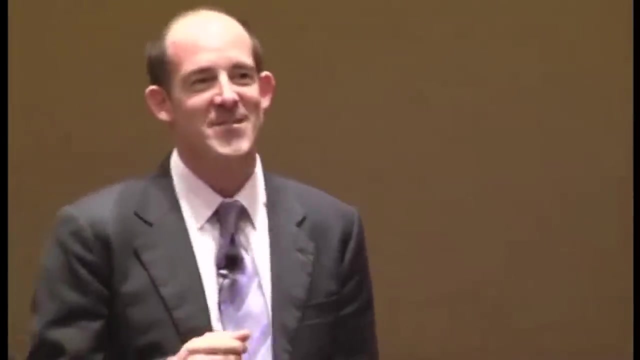 ** Hanif puegarw: hi, I'm Connor Neal. I'm Irish, 38, much like you were before you walked into this room. **. how do you get people to engage with you when you're networking? say, in networking, the best thing you can just walk up. I think we know someone in common. try and walk away. 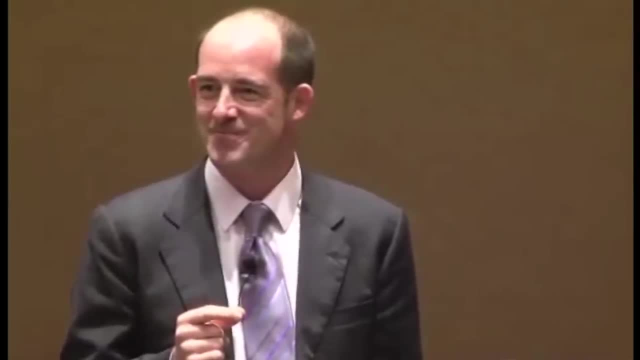 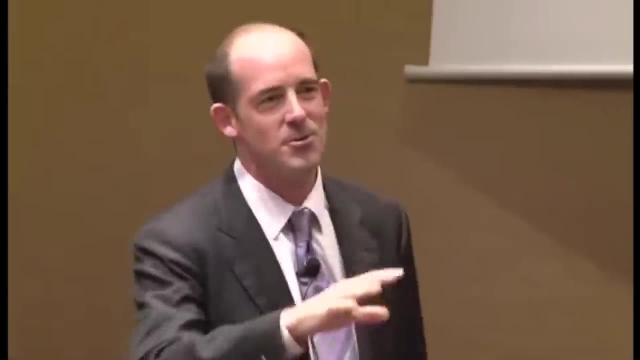 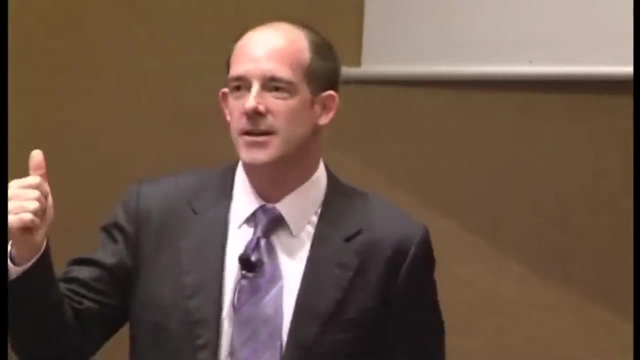 when someone comes up and says that to you. hopefully you've done your research so you do know that you've know someone in common. but with LinkedIn you can find out who knows who on anyone you want. how to start a speech first way with a question that matters to. 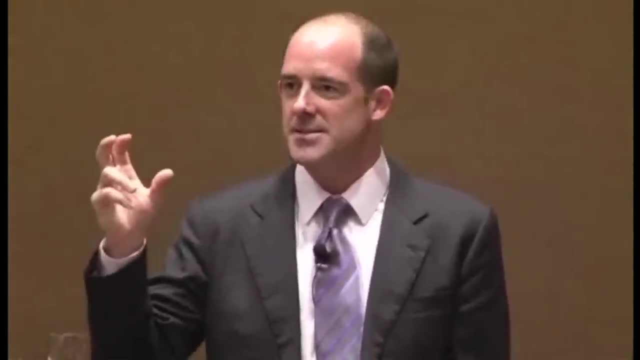 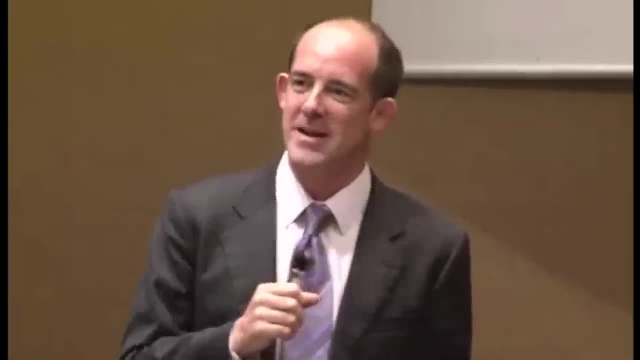 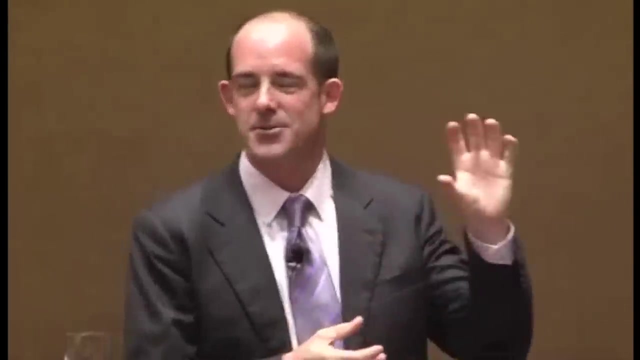 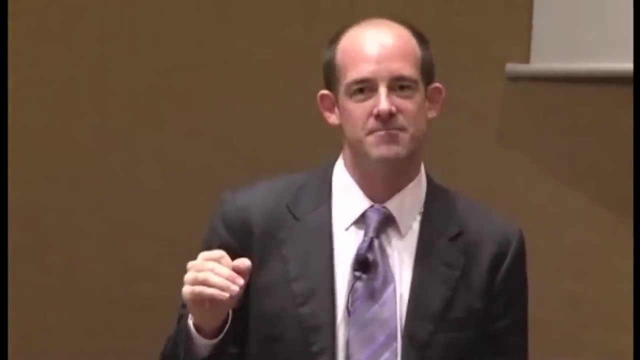 the audience. how do you phrase a problem that the audience faces in a question? so that'd be the third best way of starting a speech. the second best way of starting a speech is with a factoid that shocks: there's more people alive today than have ever died. more people alive today than have. 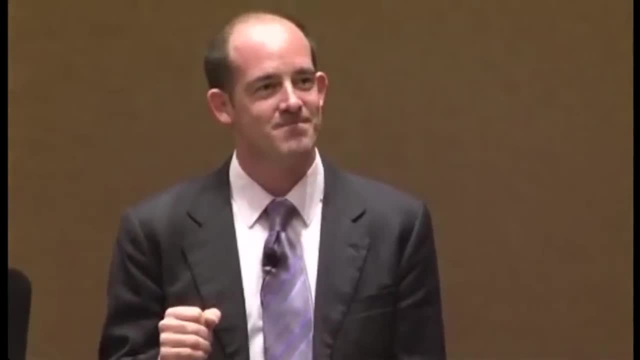 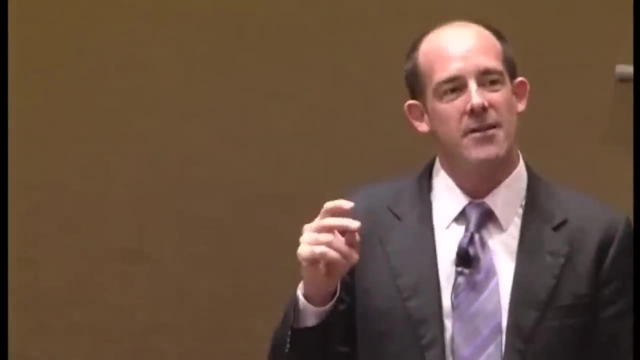 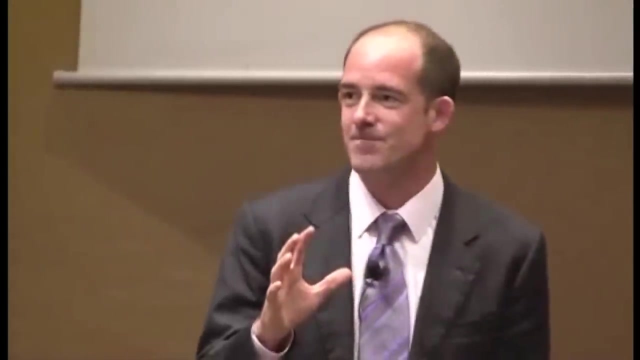 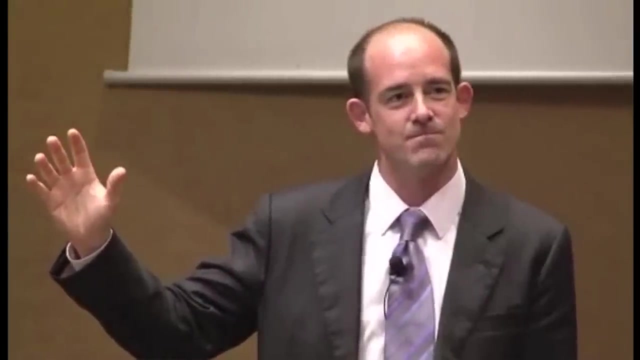 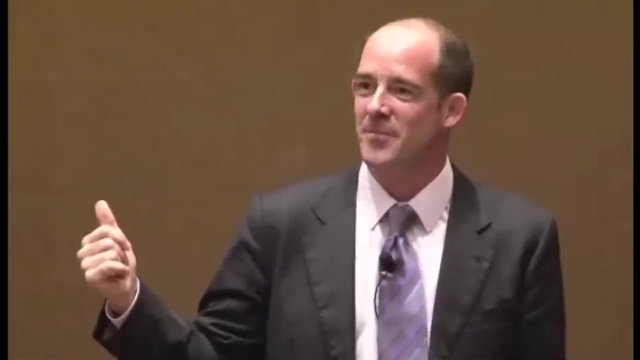 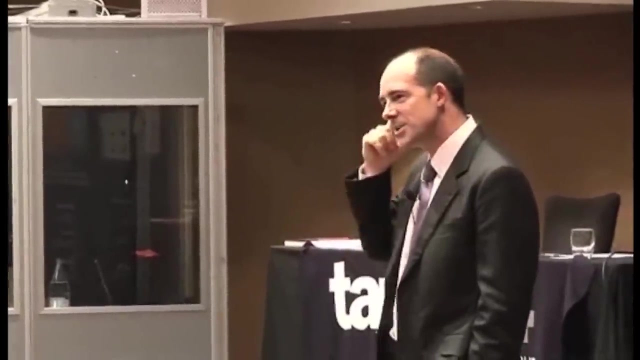 ever died. there's a lot of speeches that can follow on from there. every two minutes, the energy reaching the earth from the sun is equivalent to the whole annual usage of humanity. all the energy, all the cars, everything moving, all the lighting, all the air conditioning of the world in one year is equivalent to two minutes of sun. does that change how you? 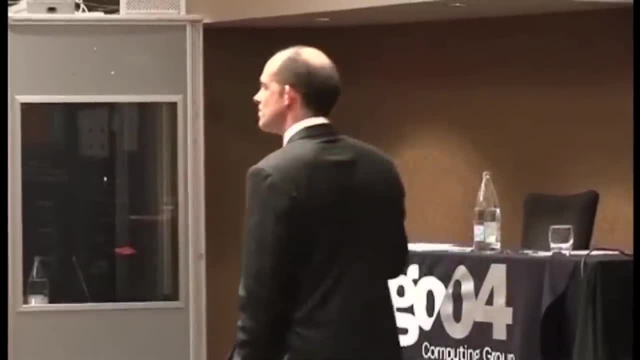 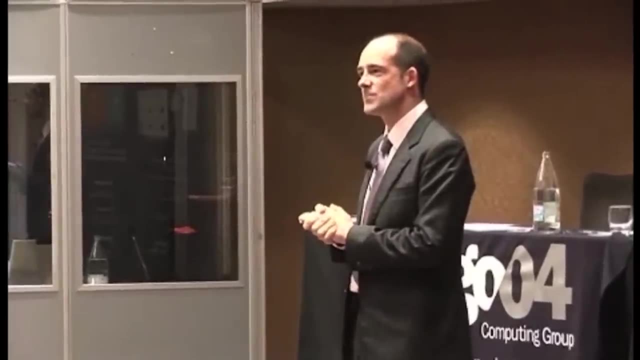 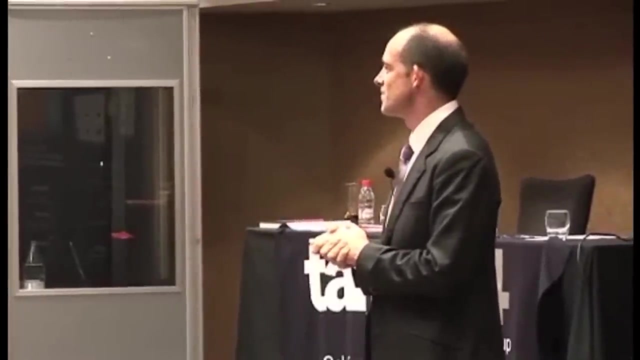 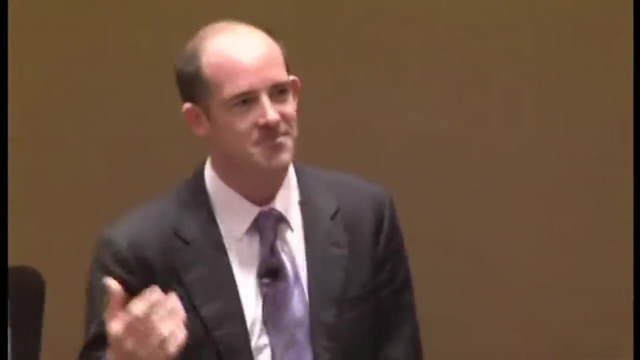 think about energy. so what's a fact that shocks the audience into? into rethinking, rethinking, and Google has transformed your ability to get at these facts. given two or three minutes, you can find out one, whether anything I've said is true, but you trust me because I looked. 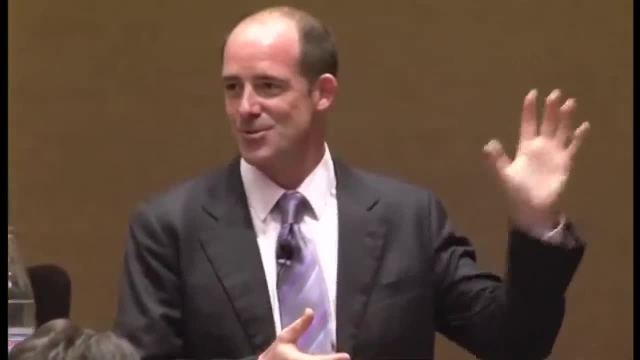 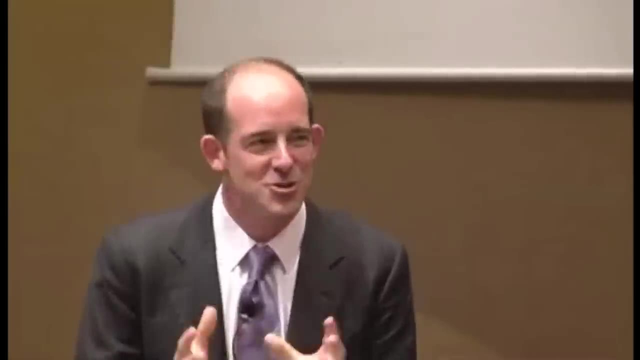 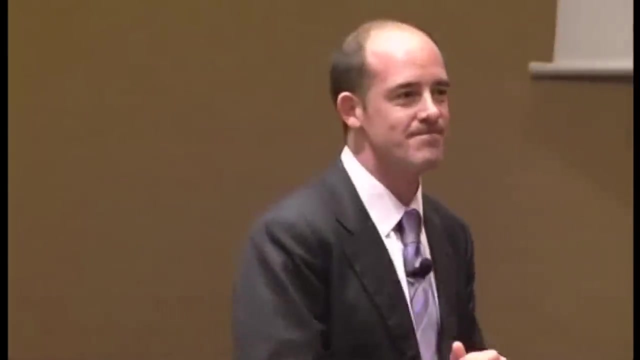 the part and I'm from the essay. those are in fact two true facts. I usually get someone come up to me and are you sure about? how do they measure dead and alive? but it's true. I'm sure of the fact that you may swear by all the things you think about the fact that you were 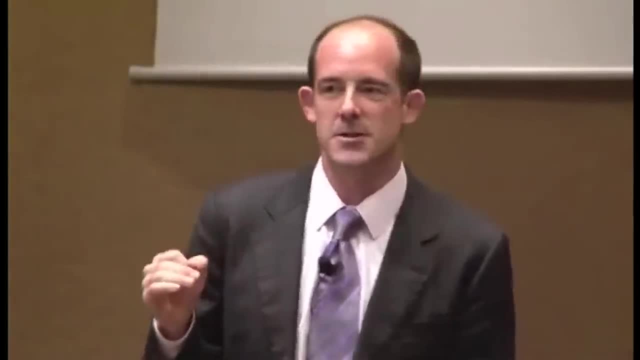 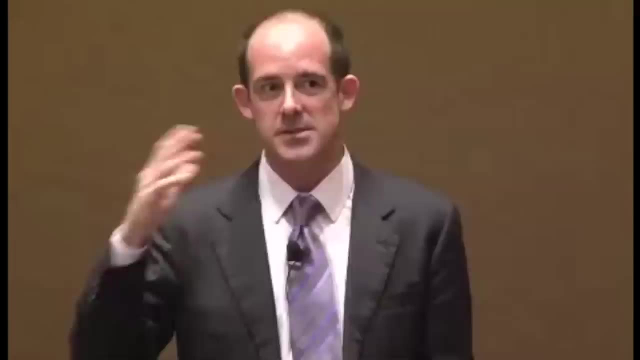 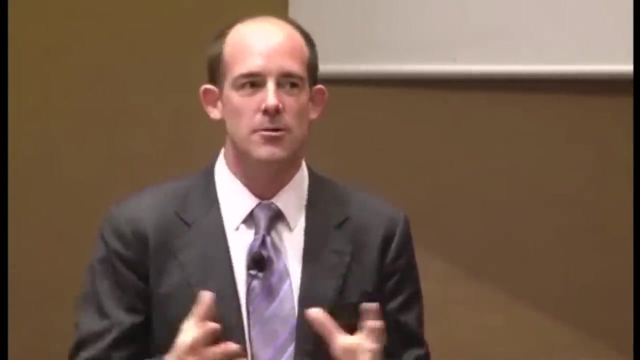 more than only one or more. you know you can't figure out what nobody else is or saying in the book. I don't know if it's true for everybody. it's actually very clear that it's not true. we're going to start a speech, but the best way to start a speech and the way that I hope all of 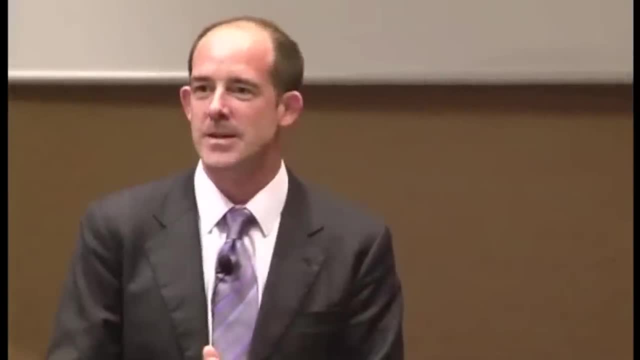 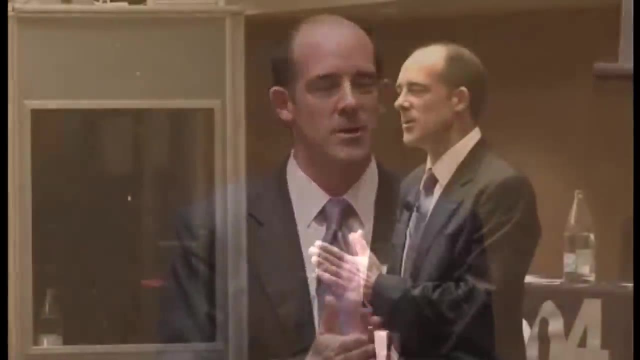 you use from now forward is the same way we start a story to a child. now how do we start a story to a child: Erase una vez once upon a time. and what happens when you say once upon a time? I can tell you what happens when. 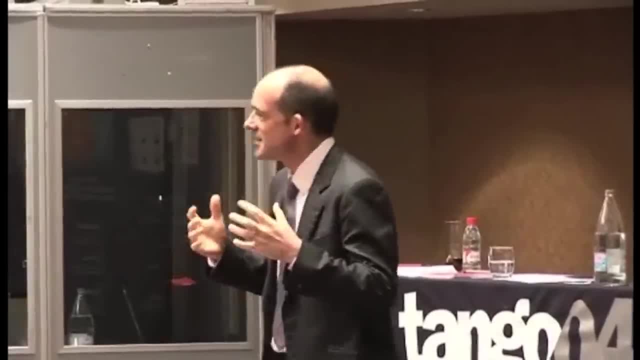 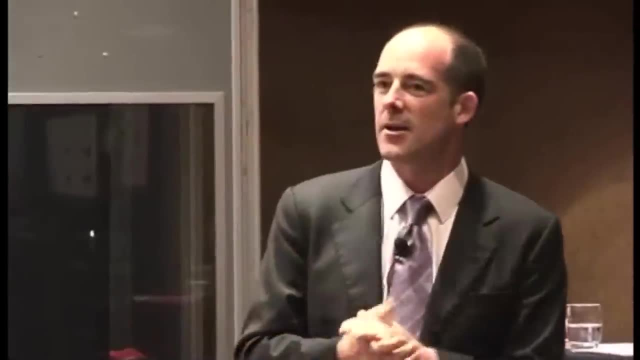 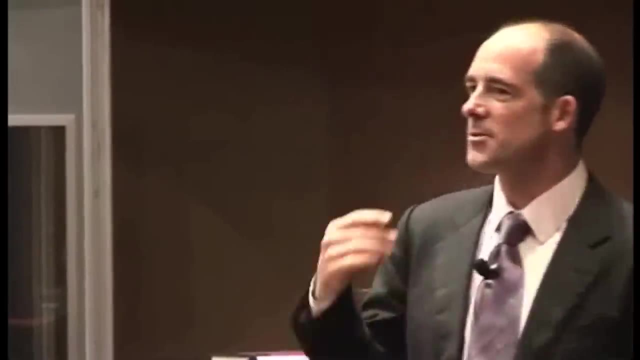 I say once upon a time my daughter leans forward, gets ready to hear, engages, and we were all trained as kids to know when a story is coming. we also know when a teacher is about to deliver a 40-minute boring lecture. that has no impact on our 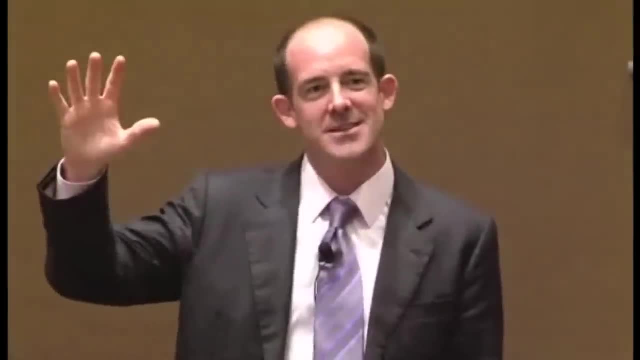 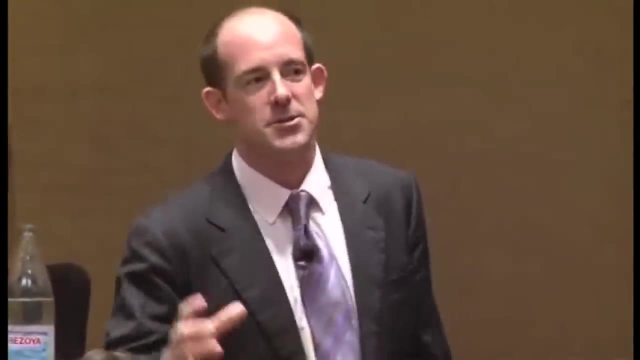 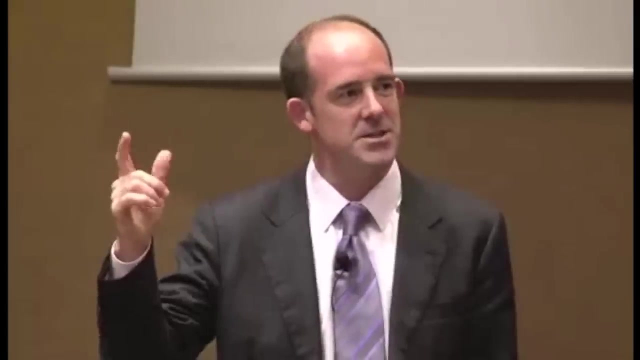 lives. but in business you don't hear Jack Welsh saying once upon a time, Steve Jobs doesn't start his speeches once upon a time, so that there's a grown-up way of saying once upon a time. and if you listen to the conversations that are interesting around you at a dinner table in a networking event, if you listen to 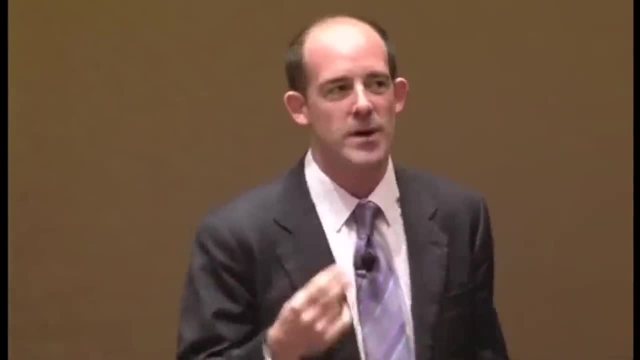 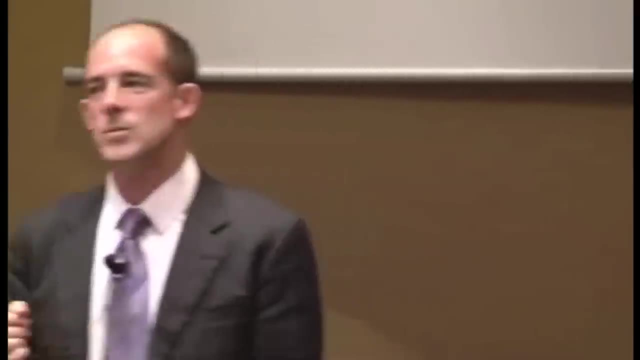 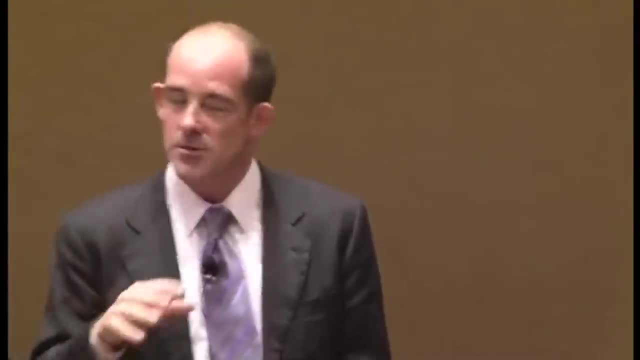 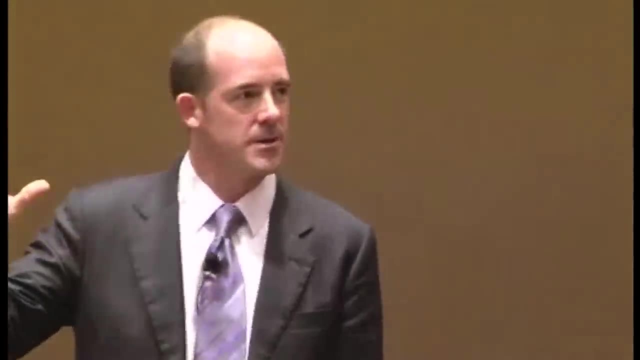 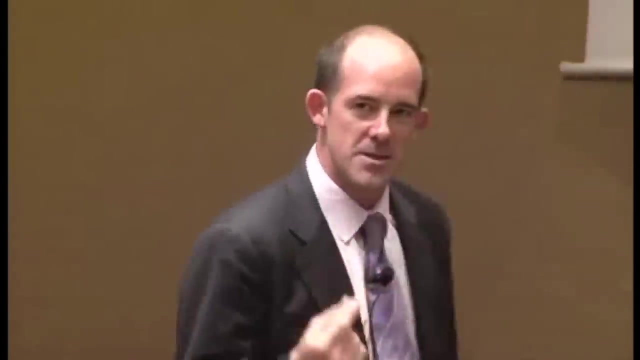 stories as an adult is. in October was the last time I was in this room. there were a hundred and twenty people in the room and I was having a little conversation with one of the world experts on public speaking and he said something to me. he said something to me that's had me thinking ever since. he said: 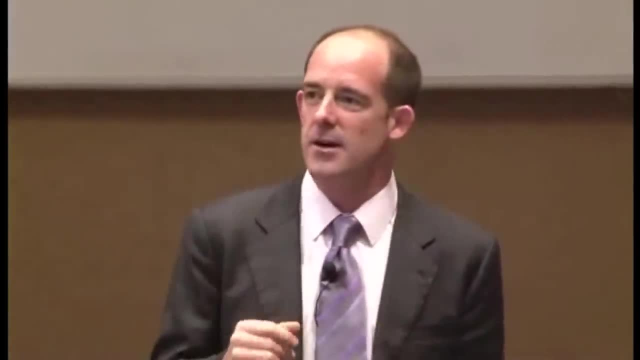 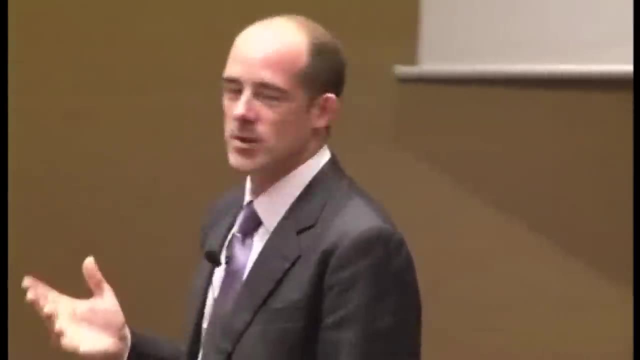 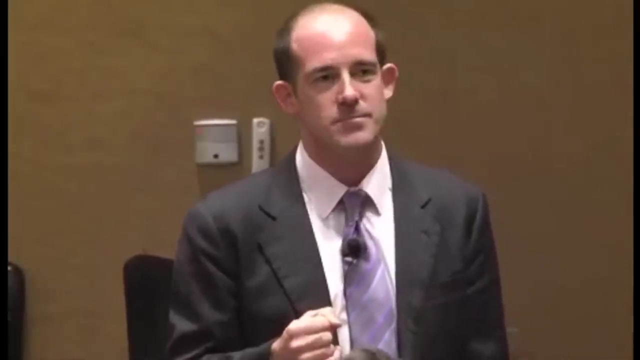 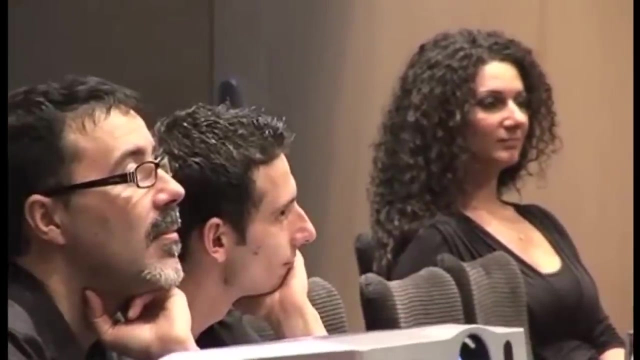 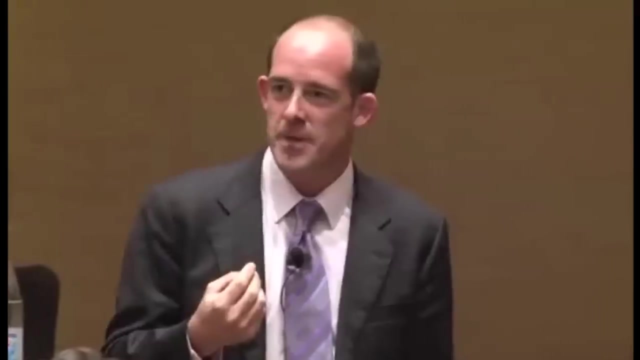 something to me that changed what I think about what's important in speaking. now I can pause for about 30 seconds, two or three minutes, and you want to know what he said. so in speaking in sales, we assume self-interest. so if you can tell a story from your own life that connects you to why this topic is, 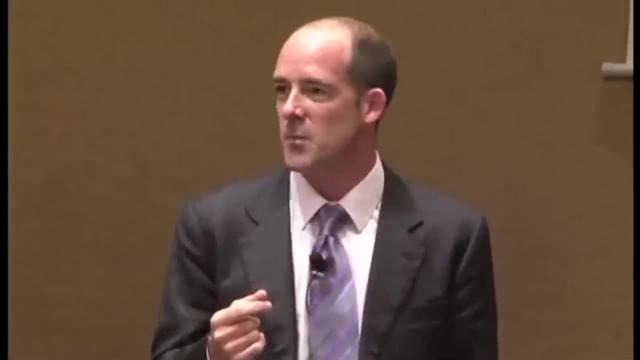 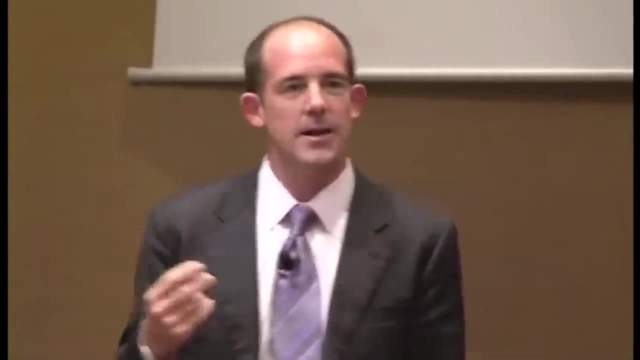 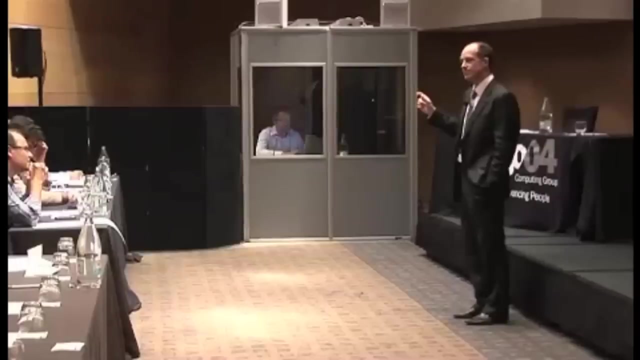 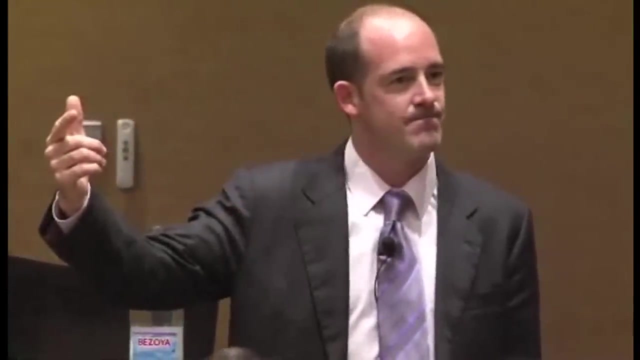 important to you why you first joined the company, when you first saw someone benefit and you saw how their life was changed, and I think here exploring what quality of life means for you in your business. how do you affect quality of life for a customer? because that's where the